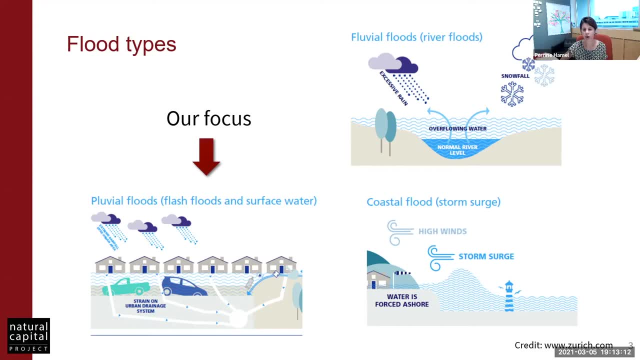 And the second type of flooding is coastal flooding or storm surge, And this is essentially due to large waves of storm surges that reach the coast where people live. So this is a second type of flooding, A type of flooding coming from the ocean or from a lake shore. 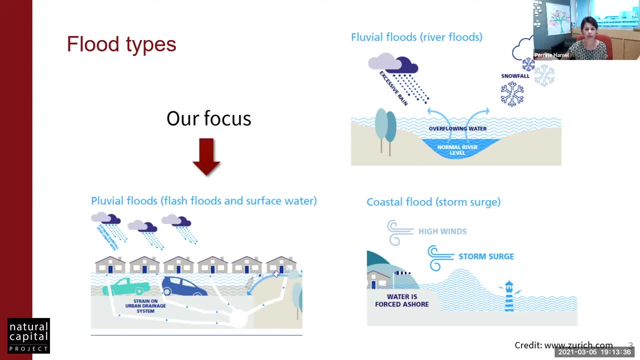 The third type of flooding is fluvial flooding, which can be flash floods when there's very intense precipitation, And, more generally, fluvial or surface water flooding, And this is actually the type of flooding that we are going to focus on today. 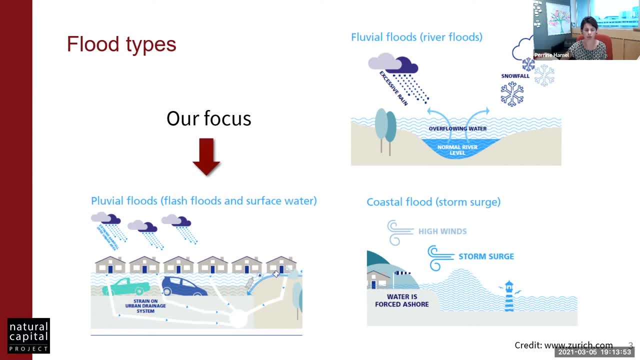 Essentially when there's a lot of precipitation in a short amount of time and either the soil is saturated or they reach the infiltration capacity, which means that there's too much water produced at the surface of rural or urban areas And this leads to local flooding. 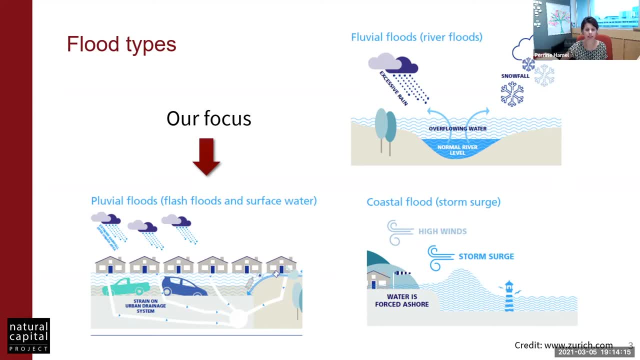 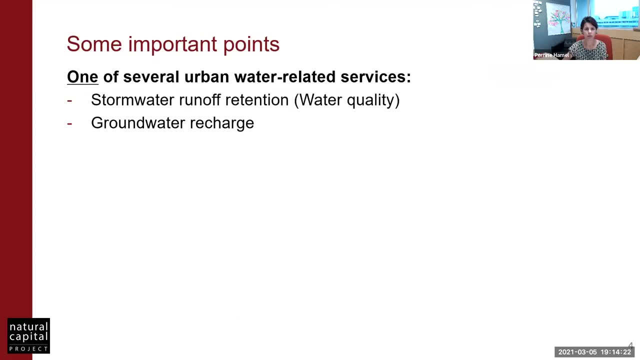 So, again, this is the third type of flooding that we're going to focus on and that the model is designed to represent. So some important points about the flood. First of all, the flood risk mitigation model, And I want to highlight that it's one of several urban water related services. 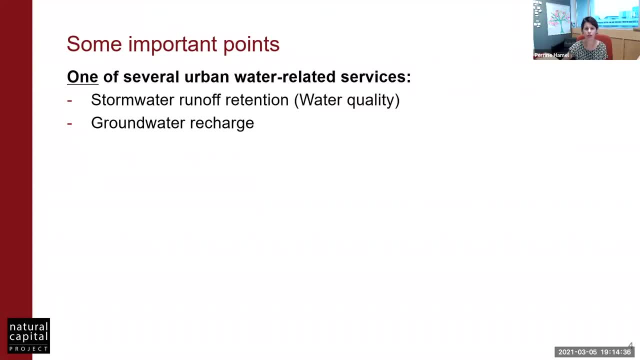 And to understand where it fits in a broader picture of ecosystem services. And so other water related services include stormwater runoff retention over longer timeframes, And this is important for water quality as well as the long term water cycle and urban watershed. So the difference between the model we're looking at today and that one is that we are today looking at extreme events. 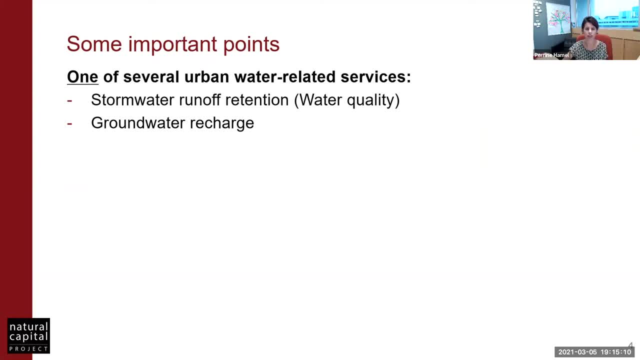 or storm events, when there's a large amount of precipitation for a single event. The other one is more for long term and water quality questions. The other related model is or service is the groundwater recharge service, which is essentially looking at how much the groundwater is recharged through infiltration in pervious areas. 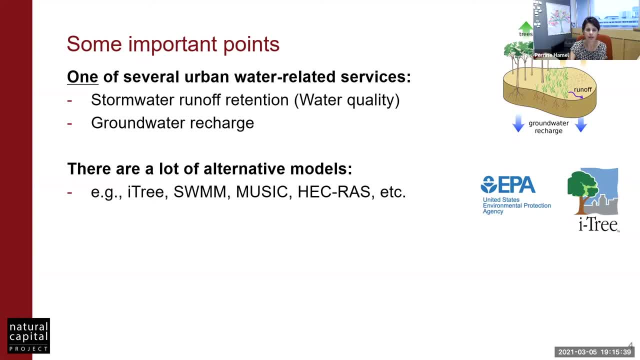 There are a lot of alternative models and that's the second point I wanted to make. that's important. Some of them, you may or may not know, called iTree, which also looks at several ecosystem services, SWMM- the stormwater management model. 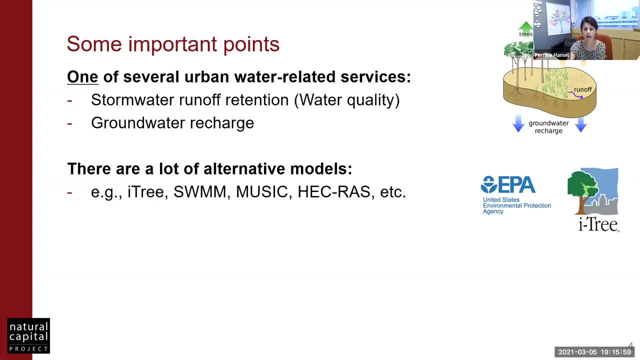 MUSIC, HEC, RAS, other hydrologic or hydraulic models that are essentially designed to represent how water flows, in that case in urban watersheds. So it's important to remember that INVEST is one option among many others, And very often these are the modeling options. 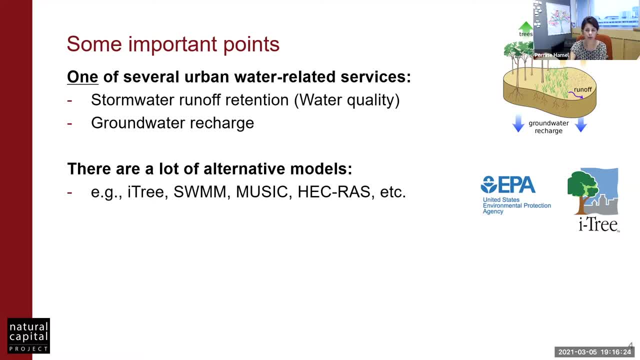 Would be more appropriate if you have a strong focus on this- urban water related services- And that's because these models are more sophisticated and will allow the user to reach higher level of accuracy. So why would anyone use the urban INVEST model in that case? 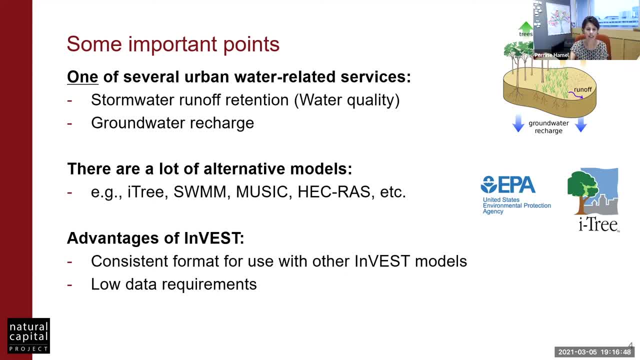 Two main reasons. One is that it's consistent in its format. the type of output and inputs are consistent with other ecosystem services in INVEST. So that's important when one wants to look at trade-offs and synergies for different ecosystem services assessments. 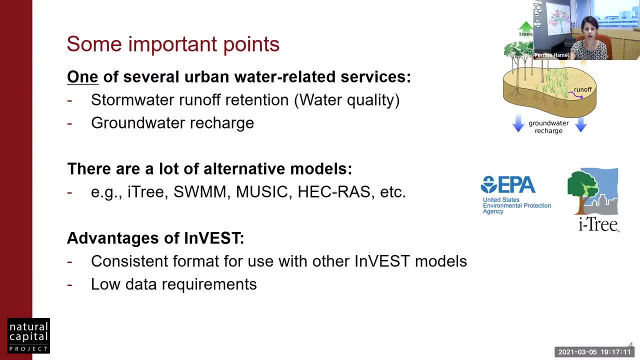 The second advantage is that there are low data requirements. Like any other INVEST model, this one was developed with data scarce environments in mind, which means that you will always find at least global data products or very easily available data products that one can use to run the model. 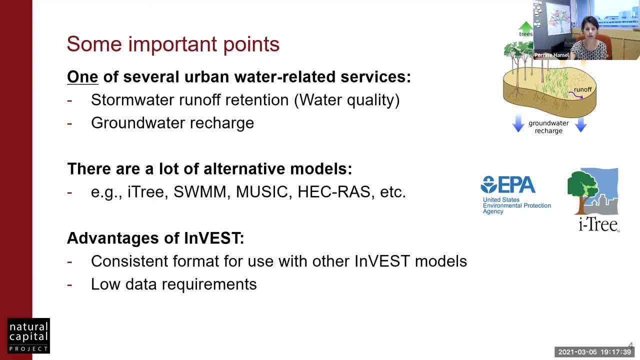 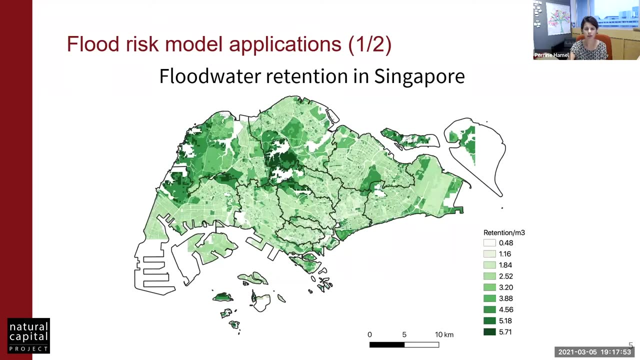 Of course, if you have better data sets- for solid data for example- it's always better, but there's a minimum product that we believe is reasonable to ask from users. So some applications just to give you a flavour of the type of model outputs. 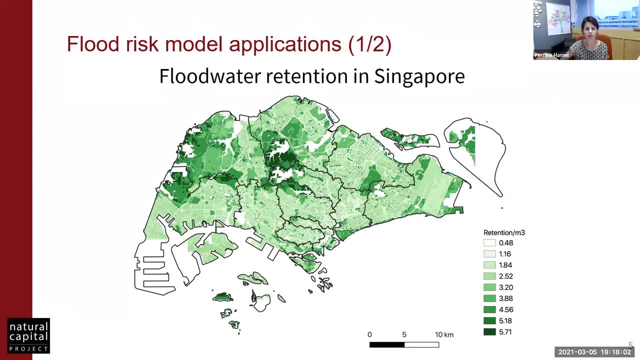 that the model produces. This is a map of the flood water retention in Singapore, So essentially looking at which areas are retaining a lot of flood water so do not contribute to flood hazard, As opposed to areas that do not retain a lot of water, in lighter shades of grey. 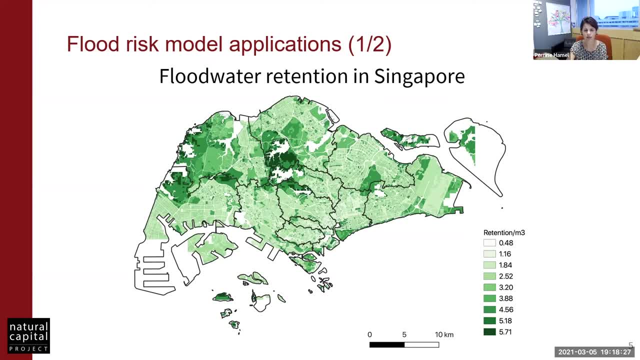 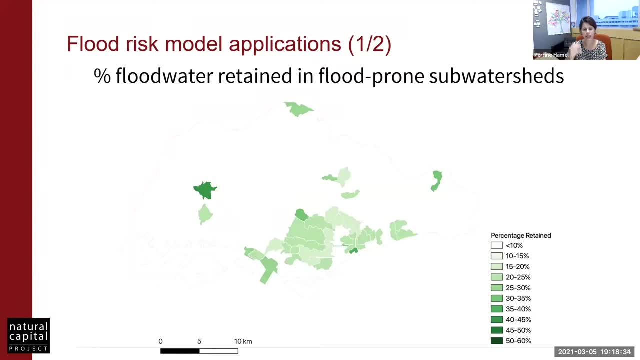 So this is an output at the pixel scale. You can see it's very fine resolution, And we can also aggregate this data at the sub-watershed level, like in this map here, And we can also focus more specifically on these areas that are flood prone. 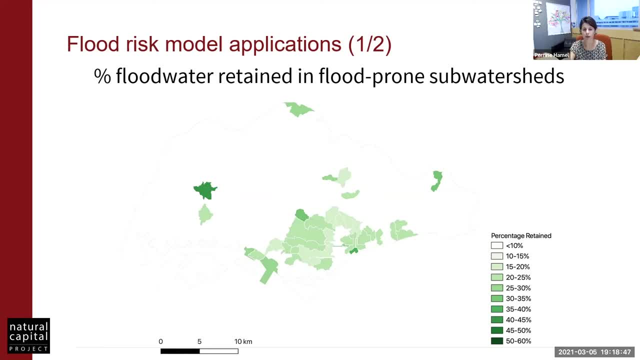 So where we know there's a risk level, there's a risk level of flooding. It's one way to determine how important and valuable this service is. This is because that's an area where there has been flood in the past And we know that it's important to protect or enhance. 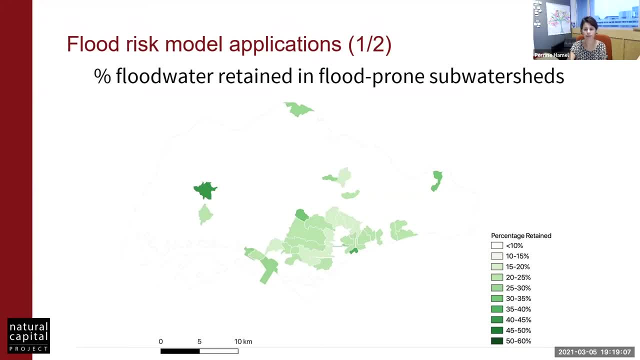 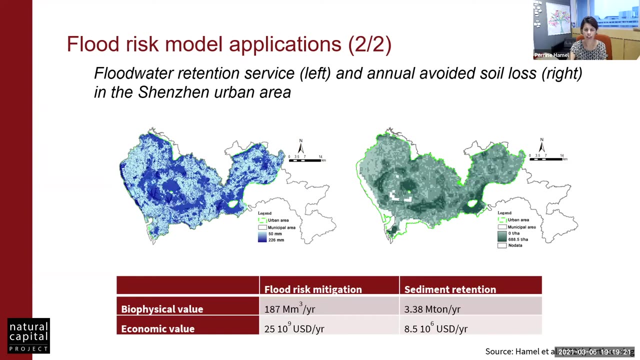 increase the flood retention service. So this is the type of map outputs that one can obtain with the model. The second example I wanted to share with you today is one in Shenzhen that some of our colleagues from the Chinese Academy of Sciences have developed with us. 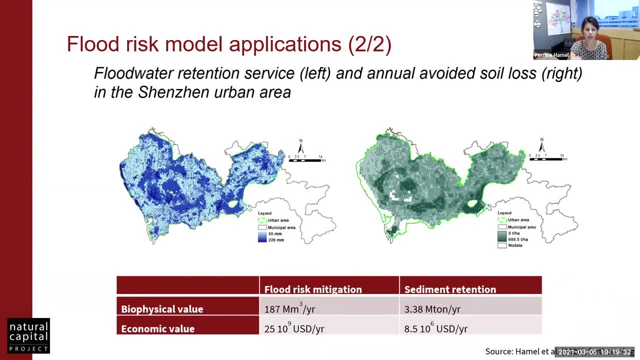 And so on this slide here, we're showing two maps: one for the flood water retention service, the one we are looking at today, another one for sediment retention, And this was part of an application of the model where we wanted not only the biophysical values, 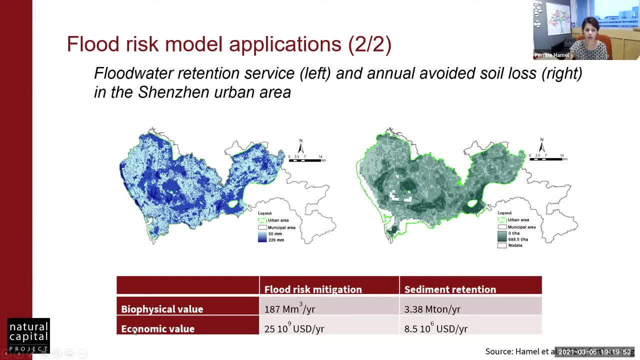 for a suite of services, but also the economic values, And this is part of a larger initiative and project looking at calculating the gross ecological product for cities and, more generally, for provinces in China. So this is another application where we can translate this flood water retention service into an economic value. 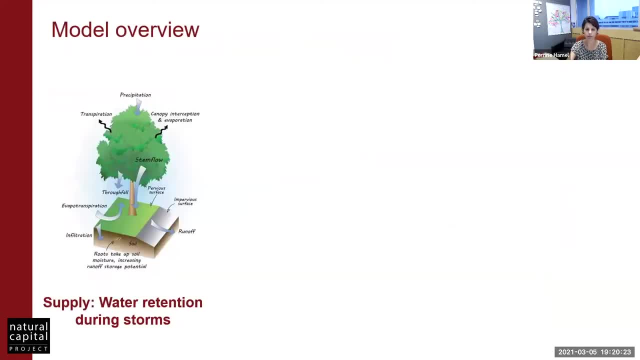 that can be used in such applications. So let's get an overview of the model to understand how it works. The first step of the model is essentially to look at the supply of the service, And by supply we mean the ecological functions that provide the infiltration and this retention service. 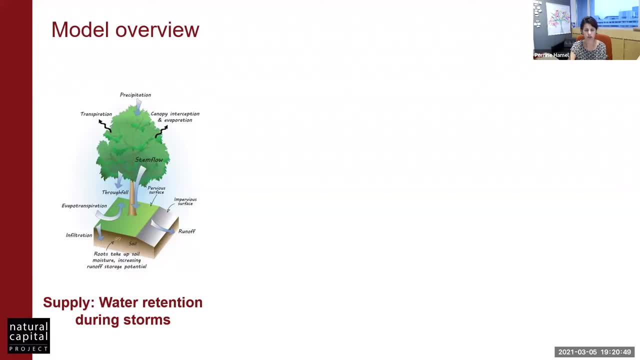 So that's essentially, during a storm, how much of this water will not be converted to direct runoff, which will increase the flood hazard? The second area or component of the model is the reduction of flood water volume in flood prone areas. So that's the connection between the biophysical component. 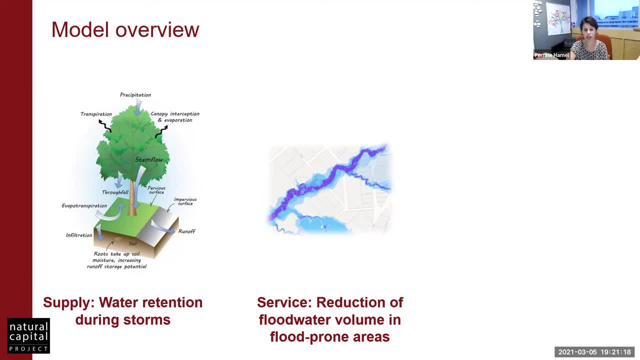 and the reduction of flood water where there's a risk, So where the value of this service is actually assumed to be the highest. And finally, there's the valuation step, which can be calculated optionally as the avoided flood damage for a flood. So that's essentially the three steps. 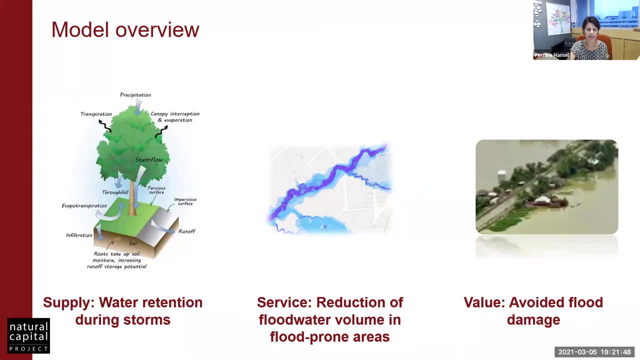 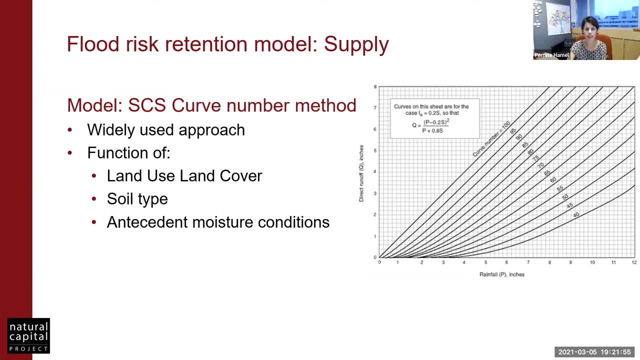 that I'm going to detail in the next slides. So for the supply, the model uses the SES curve number method, which is a widely used approach, empirically based approach that calculates the direct runoff. So if we look here at the graph in inches or in millimeters, 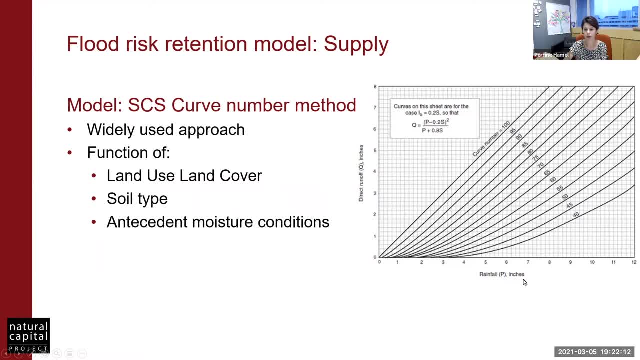 as a function of the rainfall depth- same thing in inches or millimeters- And so this relationship between direct runoff and rainfall depends on what we call the curve number. This curve number is different for different types of land use and cover, So, for example, for pervious versus impervious. 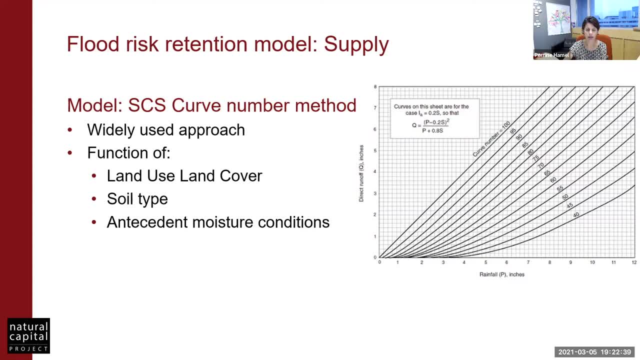 And it also depends on the soil type And the antecedent moisture conditions, which is one parameter that the model currently ignores. So, to summarize, it's mainly the land use and cover which is one of the inputs, and the soil type. 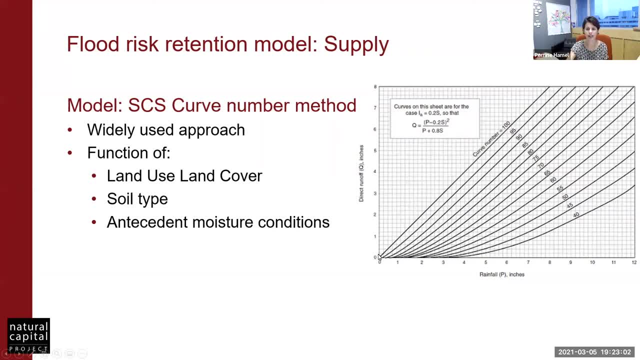 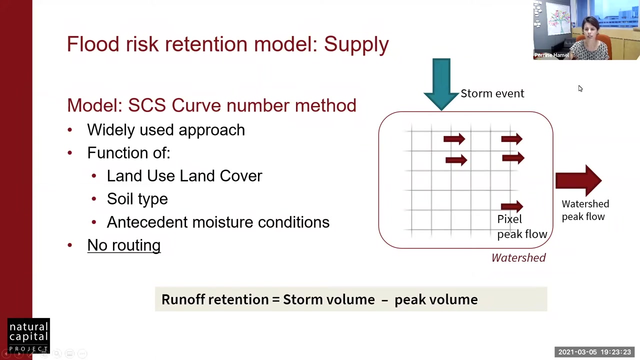 which is also a model input, as provided as a raster. So the model will use this curve, these curves, to calculate the runoff provided or generated on each pixel over the landscape, And the next step is simply to aggregate. So, for each pixel, this peak flow. 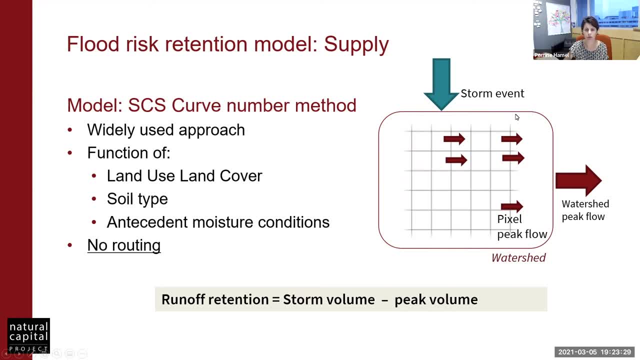 or essentially the runoff generated by the storm event is calculated, And these individual, individual pixel runoffs are summed up to contribute to the watershed runoff. And so- this is an important point for this model- There's actually no routing, which is a simplification. 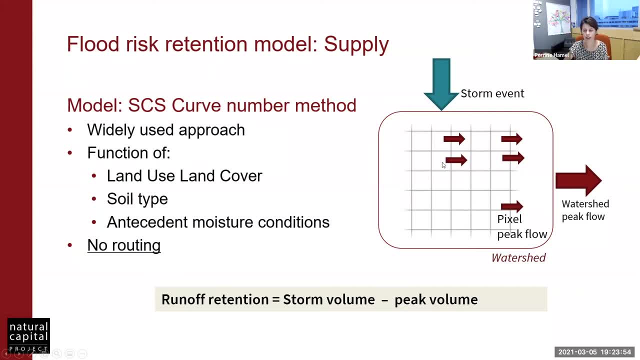 So by this I mean there's no direct routing from one pixel to another, with perhaps some possibility for infiltration, But there's essentially. these processes are ignored in the model, So it's simply the sum of all these runoffs which is acceptable for this type of model. 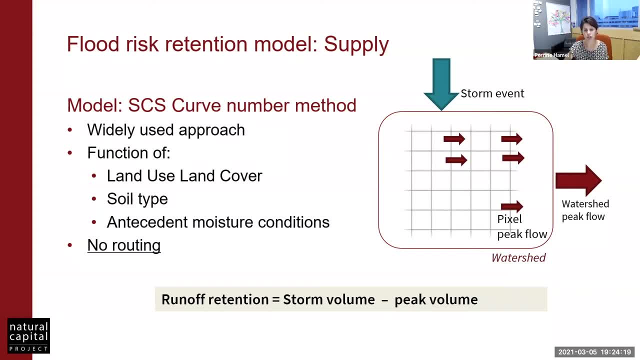 essentially assuming that everything contributes to during this launch event. So there's no timing difference between the pixels further in the watershed than those really close to the flood prone area And so and the runoff retention is simply the storm volume, So essentially all the water that this storm event. 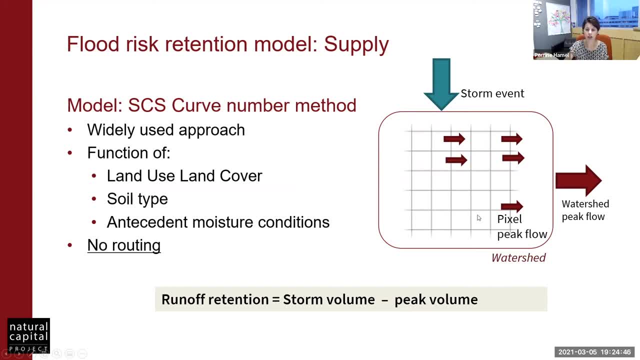 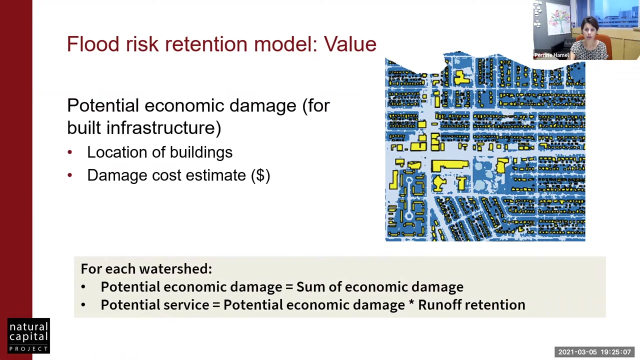 this precipitation brought minus the peak volume. So what is actually coming out of the watershed? what runoff is generated? So the difference between the two is what has been retained by some of the pixels. Next we move to the value of this service. 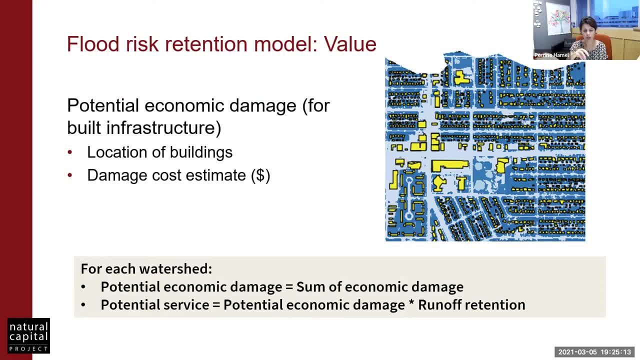 So we saw that we can focus on flood prone areas and, in particular, flood prone water sheds, to understand where this value, this service, might have the highest value. And if we do that, we can also look at the potential economic damage for flood risk. 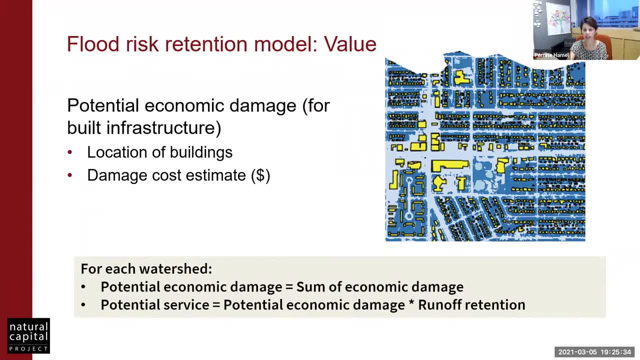 So the model? it does not explicitly look at the flood depth, It's only saying there's that much runoff that is generated, but we don't know if it's going to translate into a large or small flood in terms of the depth of the flooding. 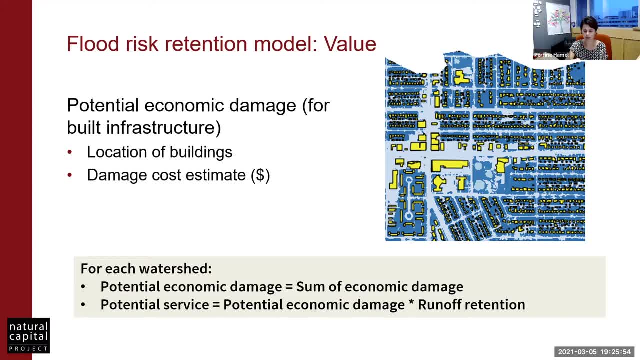 But still, if we aggregate these values at meaningful units and areas, we may want to look at what is the potential economic damage. If there is an important flood hazard in one area, the value of retention is actually highest if these buildings and the potential damage is higher. 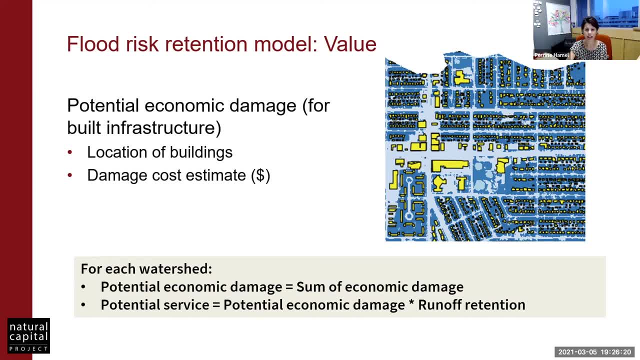 So that's essentially what the model is doing here: Looking at the potential economic damage of an area, summing economic damage for every single building that we have the footprint for, and then looking at the potential service, which is simply multiplying runoff retention and potential economic damage. 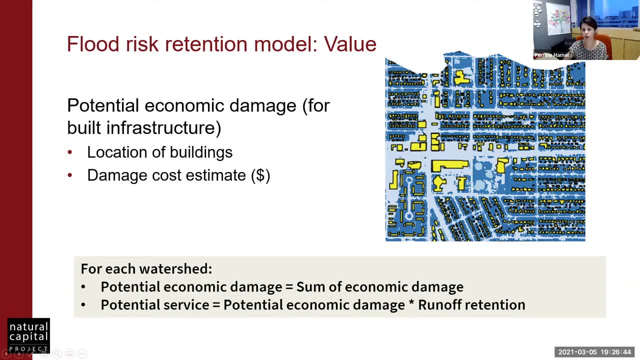 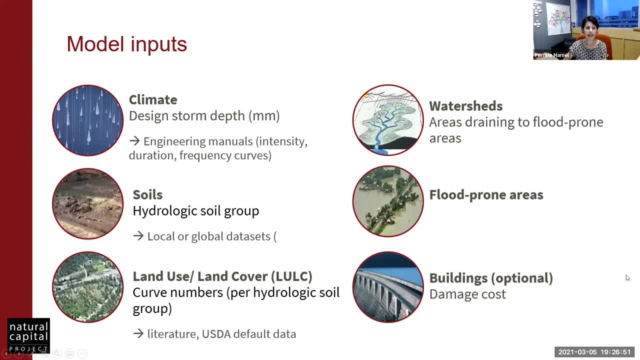 So this economic damage for all the infrastructure in an area. So if we summarize the model inputs that we just went through, there's first the climate input, which is this storm depth- And I wrote here design storm depth because often it's a choice that the model user will make. 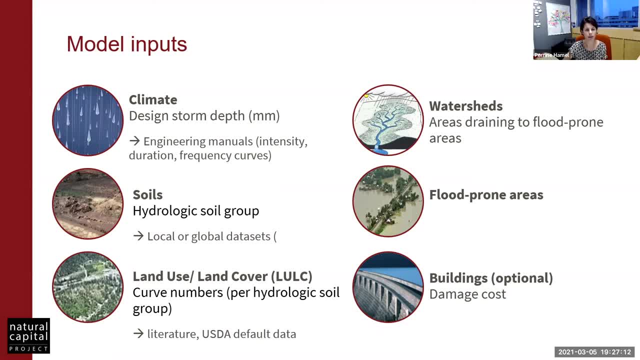 to focus on maybe a five-year return period, which is a relatively frequent event, versus a 10-year, 50-year, perhaps 100-year return. So, statistically, this is the type of event that occurs every 100 years, And these can be obtained from engineering manuals. 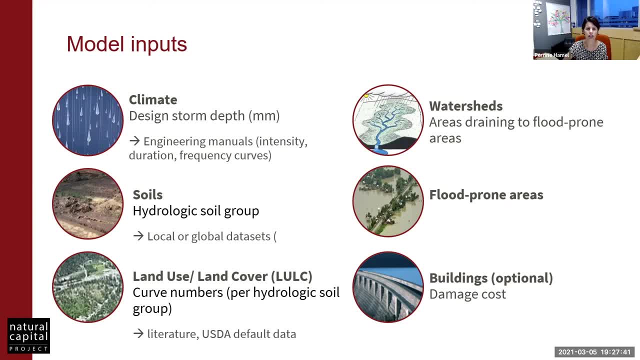 and what we call typically intensity, duration, frequency curves, essentially looking at these frequencies. So if we select a 10-year flood and then looking for a typical duration that one might select as the time of concentration, so how much time it takes for a drop of rain? 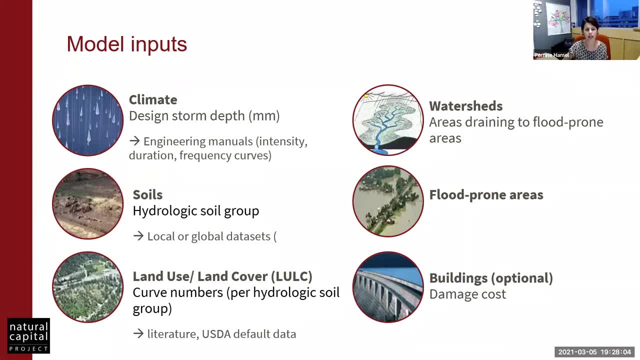 to reach the outlet of a watershed, and this could be taken as the duration. The soils data are also important, as we've seen, And so it's essentially the hydrologic soil group that we need for this model, which is a categorization of soils. 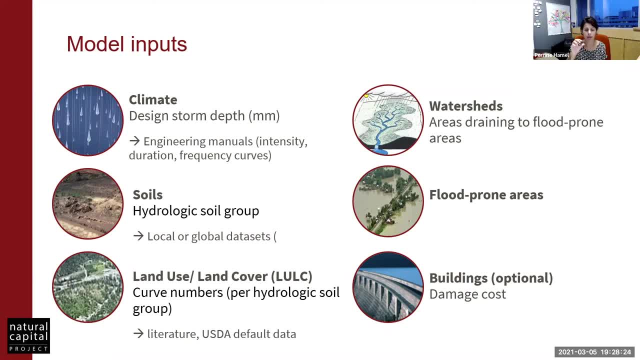 according to their infiltration capacity, And these are simply A, B, C or D, And they will be codified in the model as one, two, three, four. One for A, two, four for letter D. Same thing this can be from local soil data sets. 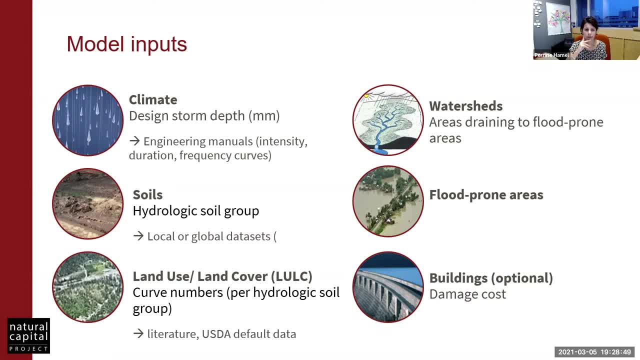 or global data sets. Finally, on that side, the land use and cover is an important input And, as part of the land use and cover, which is a raster, we also want to provide these curve numbers that I mentioned, which for each type of land use and cover. 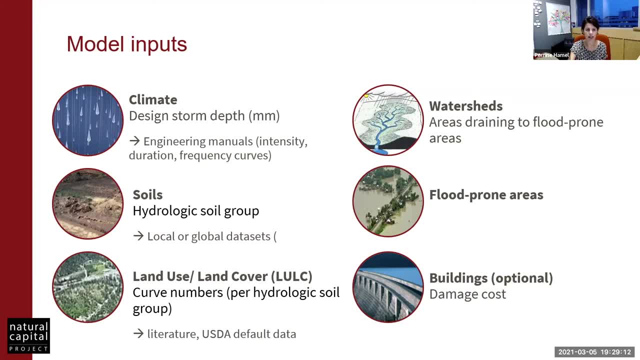 on our landscape. in the raster there's one specific curve number that's associated with it, And these curve numbers are actually per hydrologic soil group. So there's one for soil group A and one for soil group B, C and D. 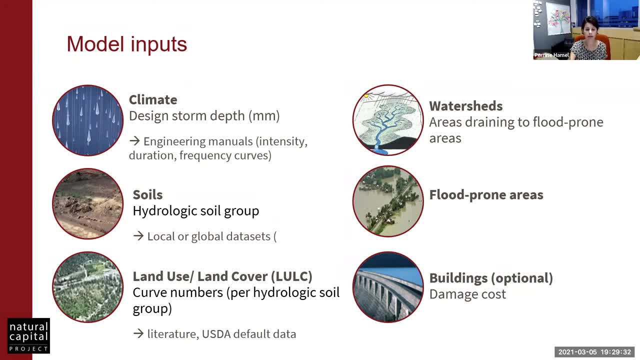 Same thing literature, because this model is quite widely used. there's often some existing studies using this data, or the US Department of Agriculture has also some default data that one can use. Other inputs include the watersheds or sub-watersheds. 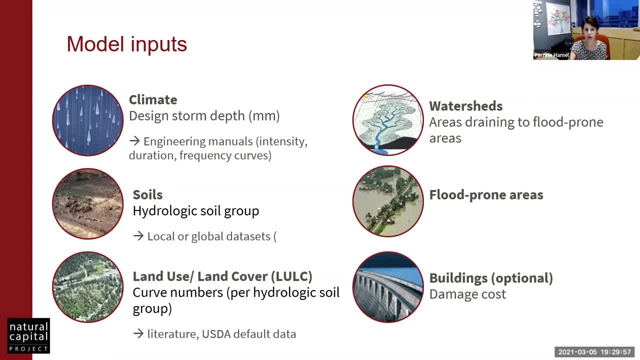 So the user can, they can define, if they want to aggregate at a coarse or fine scale Flood prone areas, which can be based on historical information and observation. They can be available from some of the local government agencies as well. And finally, these buildings and damage costs. 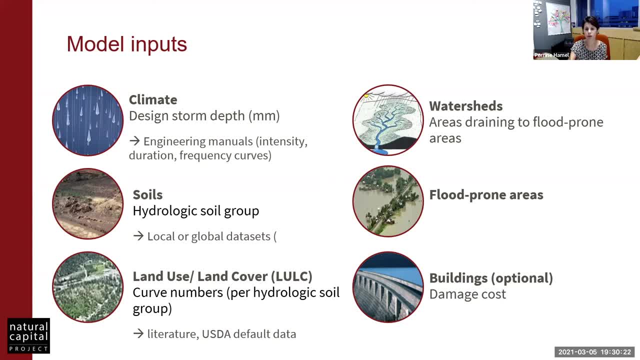 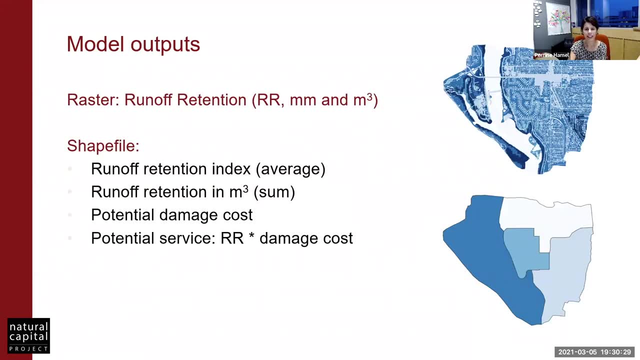 for each building, which is an optional input if one wants to go to this valuation step. So with all this input data, the model will run and produce essentially these two outputs. One is the raster of runoff, retention as well as actual runoff. 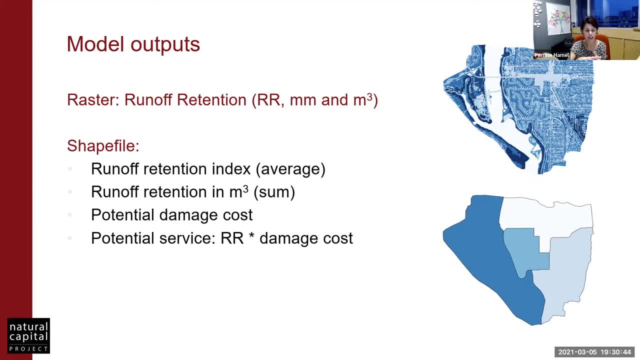 So we saw that the runoff retention is the difference between the input precipitation and the runoff generated on each pixel, And so this will be one of the outputs, as well as the runoff retention itself, And then the shapefile will aggregate these values to look at the runoff retention index. 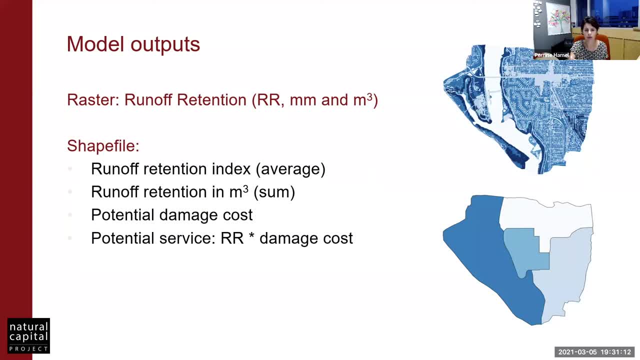 as well as in cubic meters. So both values are always as a proportion of the input, which is the precipitation, or also as a volume or a depth in millimeter. The potential damage cost as well, if the input was entered by the user, and this potential service. 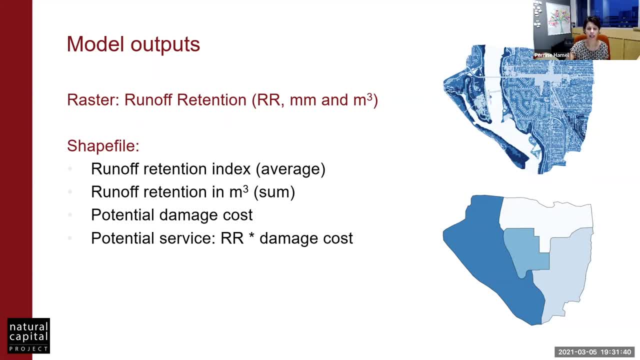 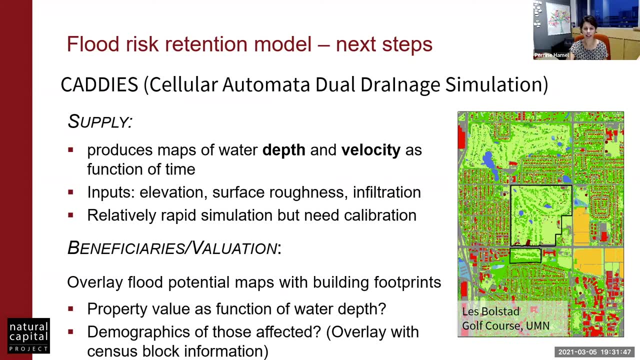 which is the product of runoff, retention and damage costs. So before going to the application and hands-on demonstration of the model, I wanted to give you a sense of some of the limitations and also the next steps. So the largest limitation of the model is essentially that we cannot look at 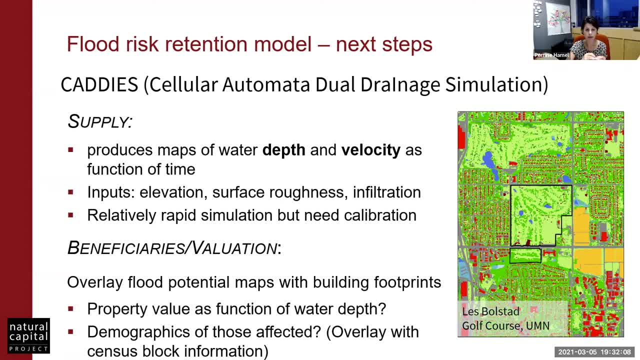 the actual flood depth that are predicted or estimated in an area. So in terms of valuation it's quite limiting. So I wanted to share here some potential next steps in terms of model development or alternative ways, using other models, that one can go about quantifying these values. 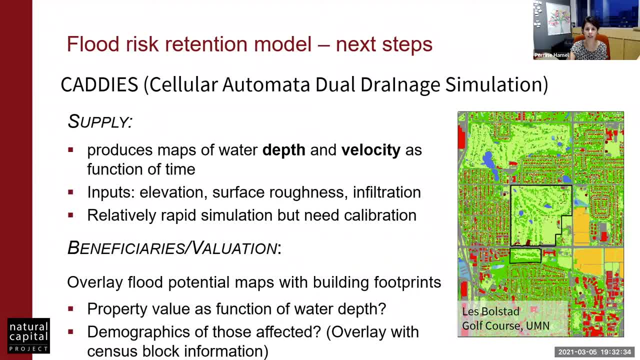 So CANIS, which stands for Cellular Automata Dual Drainage Simulation, is one model that we have tested with some colleagues from the University of Exeter to get at this question of flood depth in a spatially explicit way. So the model produces maps. 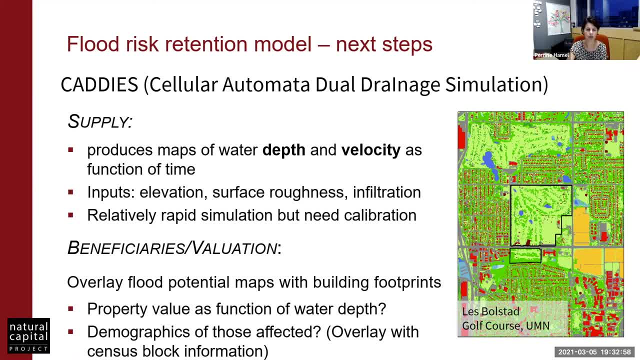 of water depth and velocity as a function of time using relatively simple inputs- elevation, surface roughness and infiltration- as a raster. So it's still much more greedy than INVEST in that sense And it produces relatively rapid simulation but needs calibration. 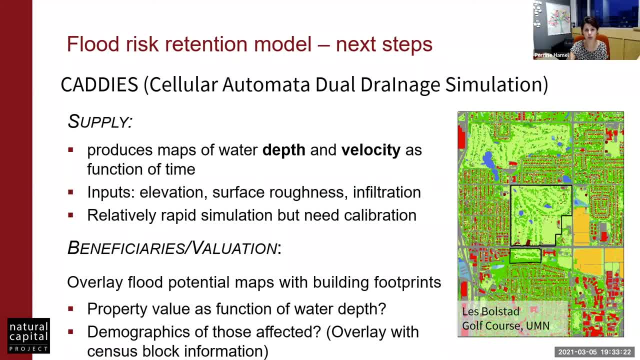 So that's one of the downsides of a lot of these more sophisticated models where you need stronger hydrologic modeling background and often need to calibrate the model. The beneficiaries and valuation step of that model can be, as I mentioned, to look directly at the property values. 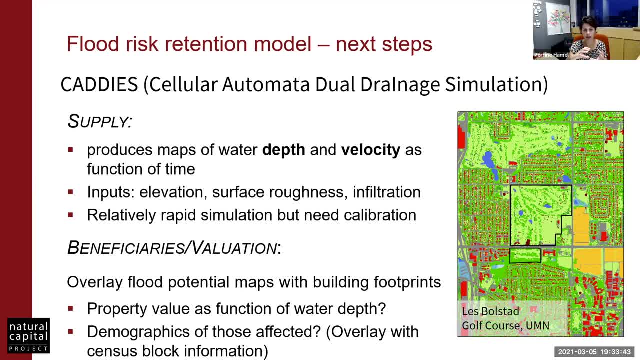 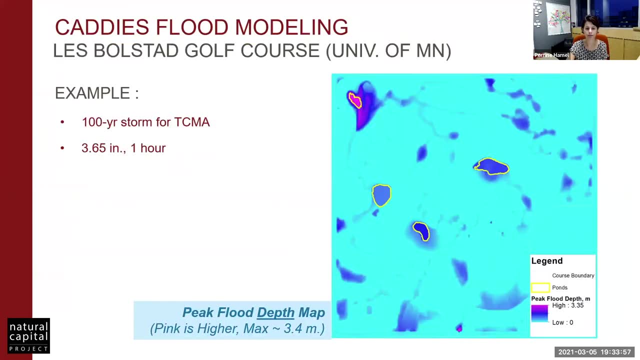 as a function of water depth And so essentially overlaying the inputs, the outputs of the biophysical model, the flood depth, with information on infrastructure or population affected. So, as an example, for a test golf course, actually in Minnesota, my colleague Ben Jenke, 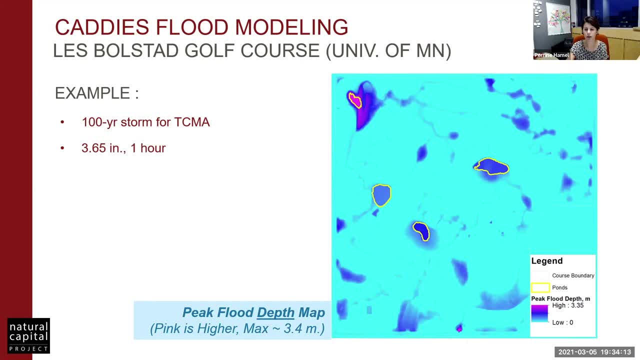 ran the model and obtained this map of flood depth here on the slide for a 100-year storm for the Twin Cities metropolitan area. So essentially all the darker colors represent higher flood depth, up to three meters, And this is the information that we can overlay. 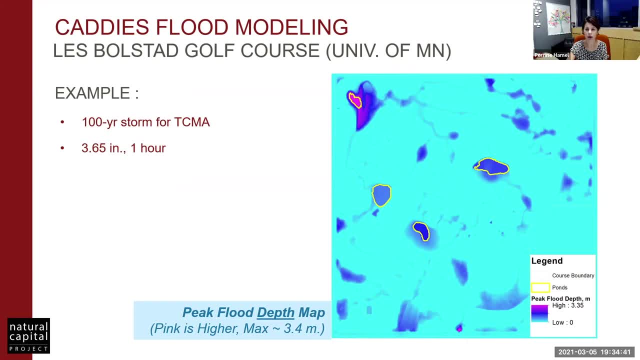 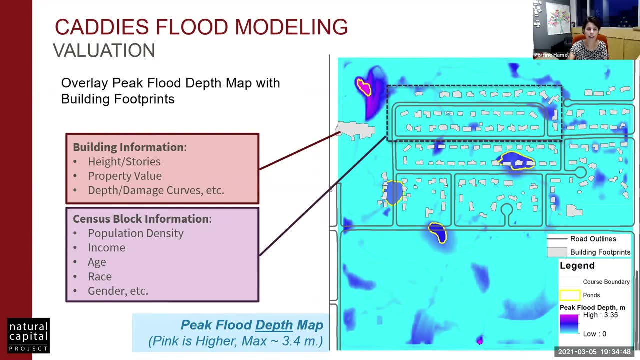 with the population of our infrastructure data. So that's what this might look like if we look at the building information in gray or information on census block. so population, income, age, perhaps more vulnerable people to flood, And so by overlaying this information, 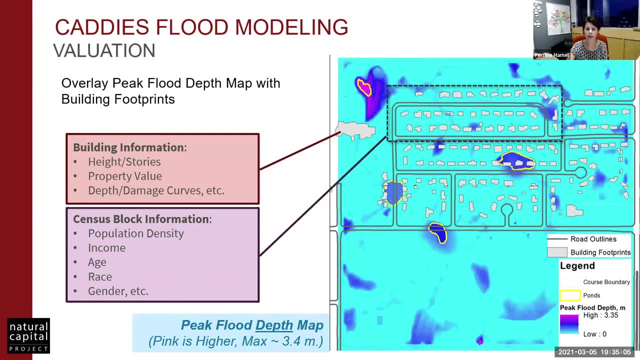 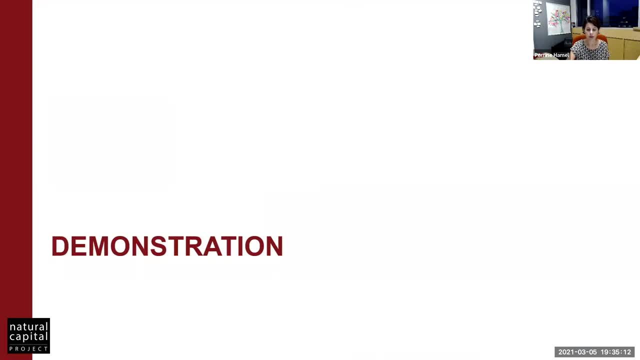 we can get a finer understanding of the value of flood risk mitigation. So that's essentially what I wanted to share with you today, And we'll just go through the live demonstration of the model to make sure that this is well understood. where the inputs go. 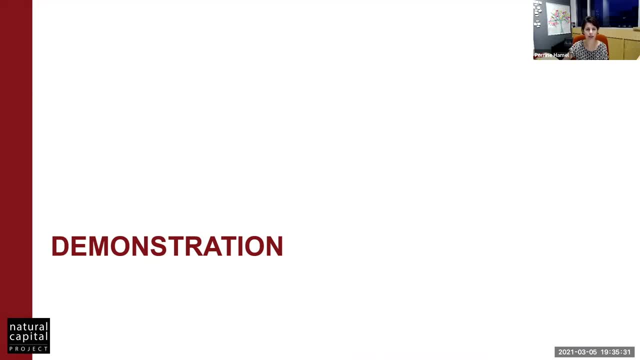 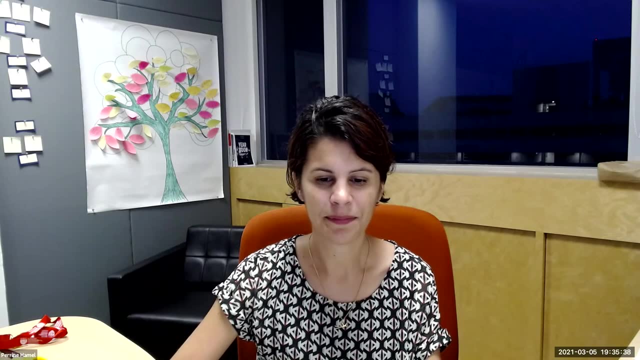 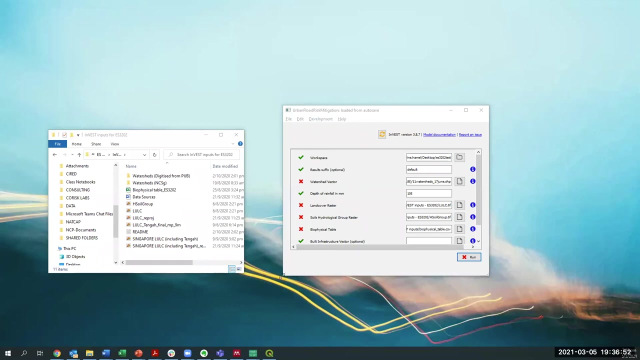 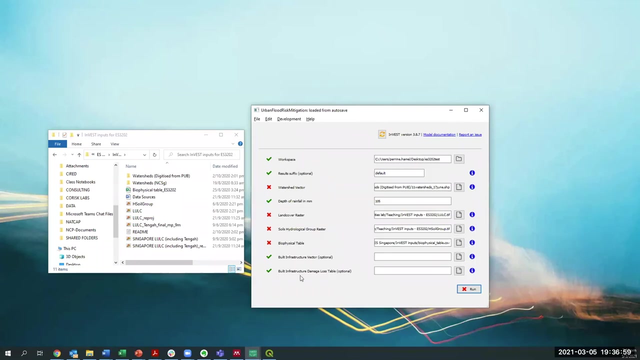 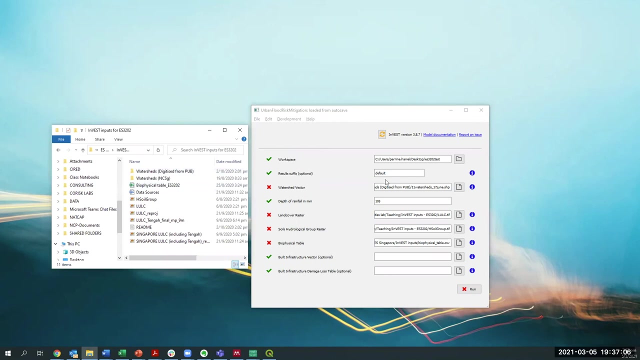 and how one goes about interpreting the model outputs. All right, So this is what the user interface looks like. So these are all the inputs for the model that we explained earlier, And essentially, running the InVEST model means entering all these data with data pre-processed. 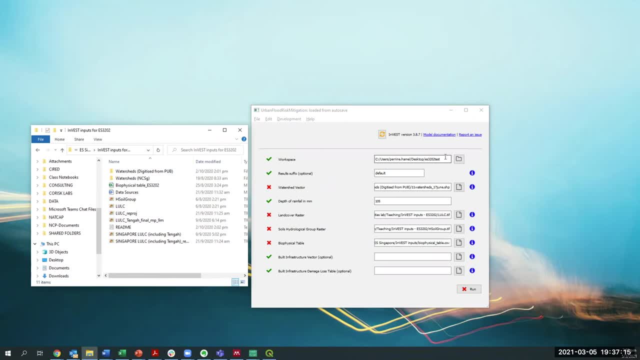 by the user and then running the model. So the first is the workspace And that's essentially anything that the user decides for where you want to write the outputs, And same thing for the results. suffix anything that's the name of the results. 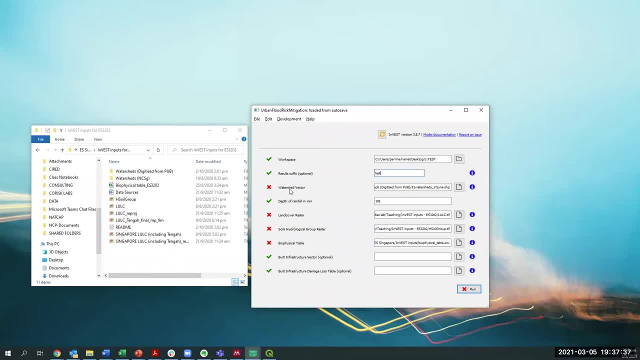 So we can call it test today. Watershed vector. So this is the watershed that is needed, or sub-watersheds. So you see that these green checks will appear as I speak For depth of rainfall. this is the design: storm depth. 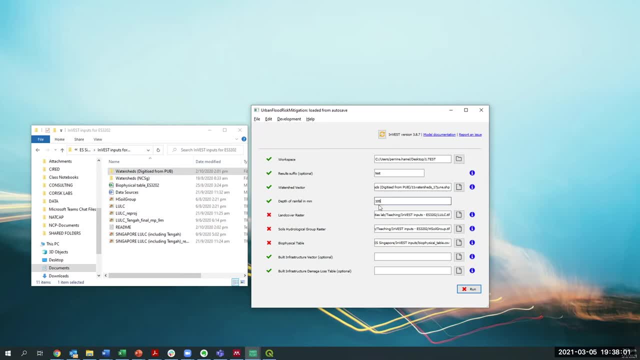 And so for Singapore we use here 105 millimeters based on the water utility guidelines, And we also look at the land cover raster. So here we're going to use a raster that we've pre-processed. So hydraulic group And biophysical table. 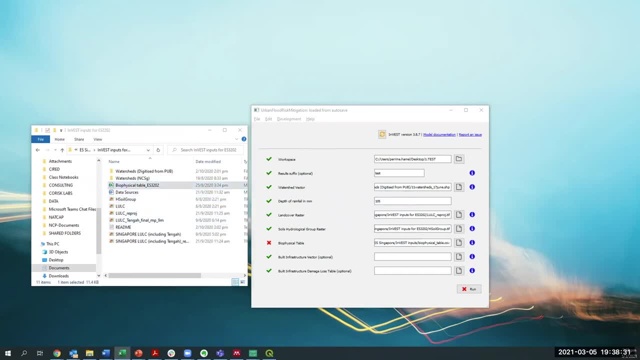 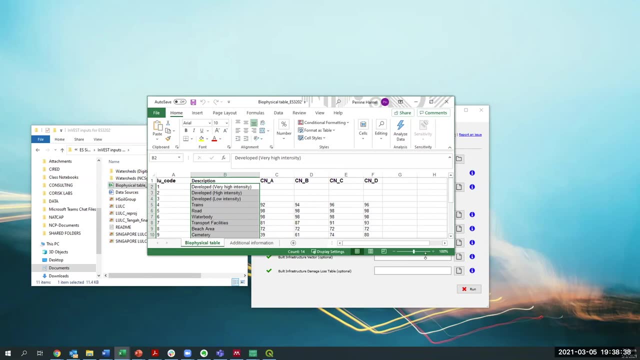 So we can take a quick look before entering this input. So this is what the biophysical table will look like. You can see that it's actually missing some information, So I'm going to use a different one. But that's the curve numbers. 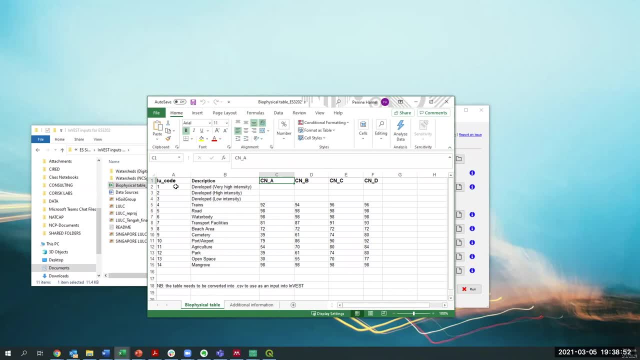 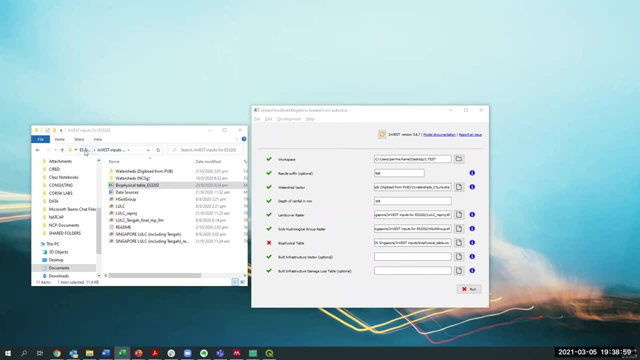 for A, B, C and D that I was mentioning for each land use, land cover code And biophysical table here, And that's about it. We're not going to use this optional input, So we just click run and wait for the model outputs. 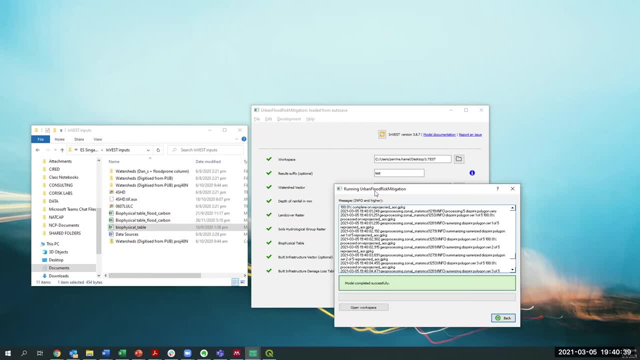 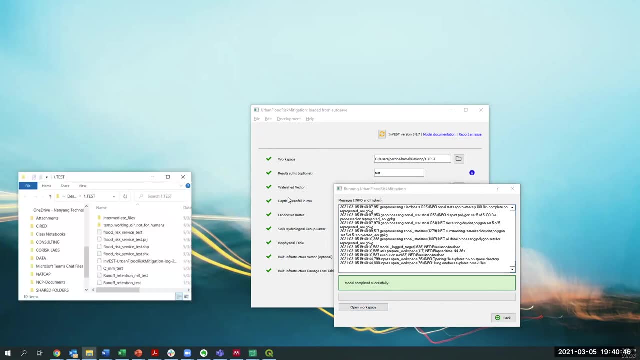 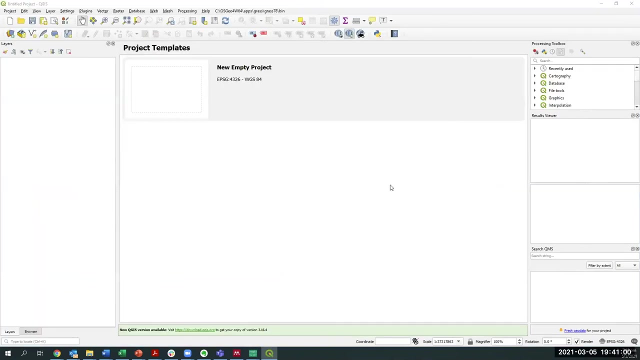 And the model has completed successfully, And so we can now check the model outputs by opening the workspace And look at the different outputs that the model has produced. So to visualize them, I will bring up here QGIS And so we can start with the shape file. 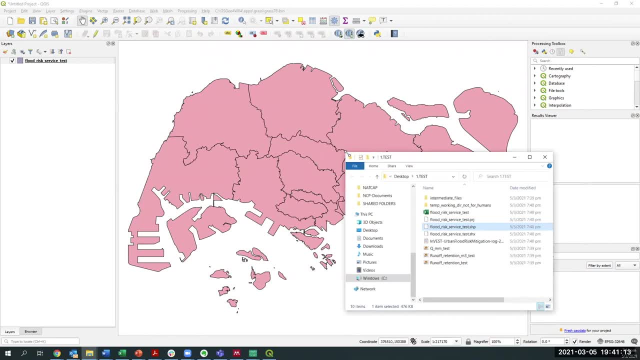 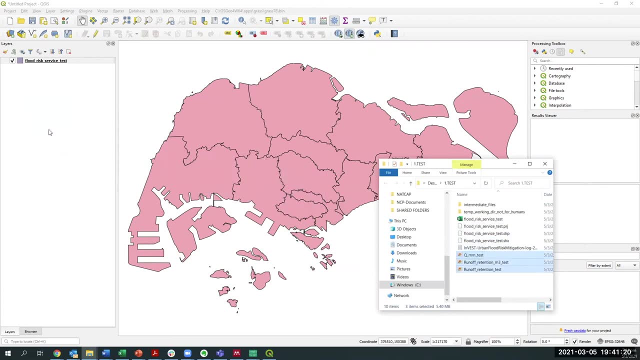 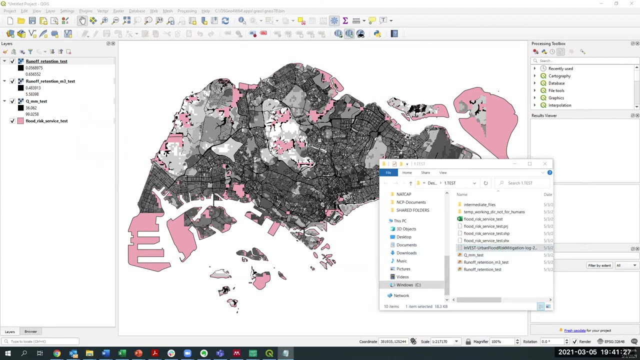 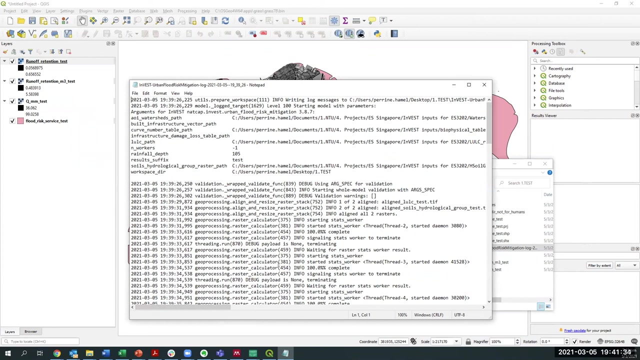 And look at the type of outputs that the model produced. I'm actually going to include them all And I just wanted, before we go into these outputs, this is also an important log file with a summary of all the inputs And also if there's any error. 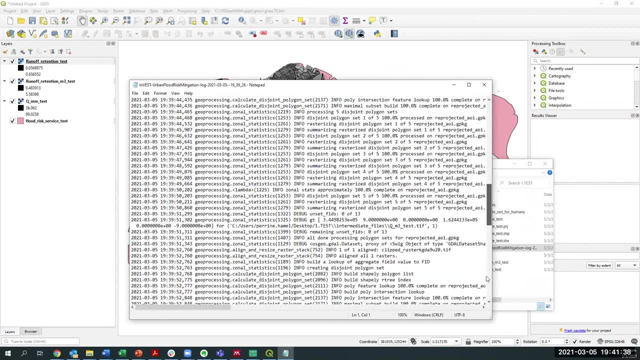 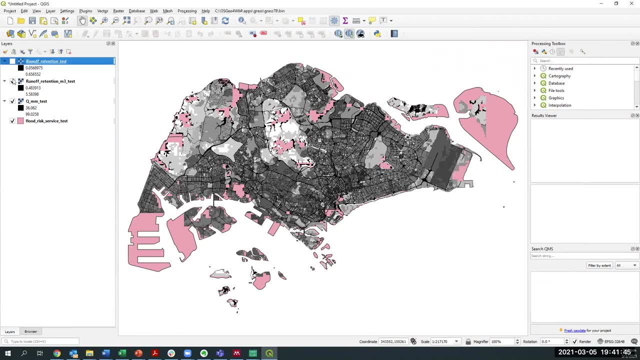 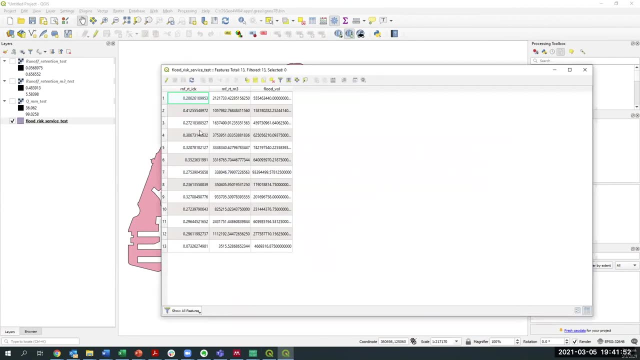 this is where you'll find some of the important information to debug the model. But so, focusing first on our shape file, we can look at. we can look at the different attributes. So the model produced the runoff retention index as a percentage and a value in cubic meters. 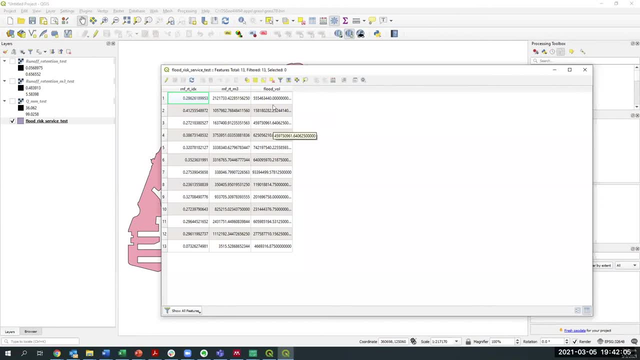 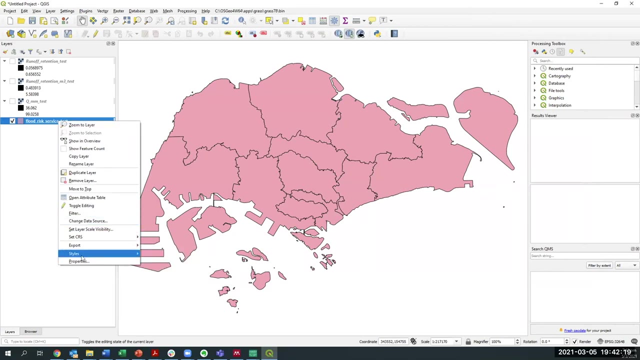 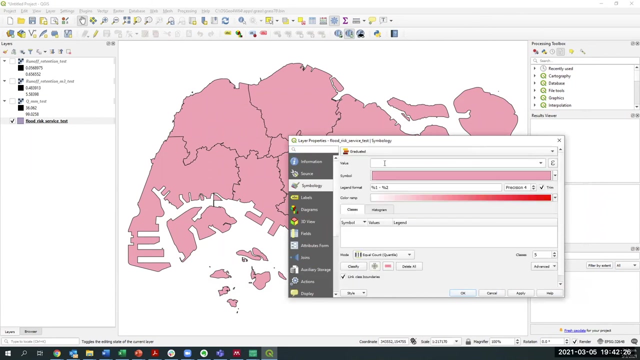 as well as the flood volume. So this is the actual runoff, total runoff, not the retained volume. So, of course, if we want to represent this in a more visual way, one might want to graduate and represent this as a function of the potential.